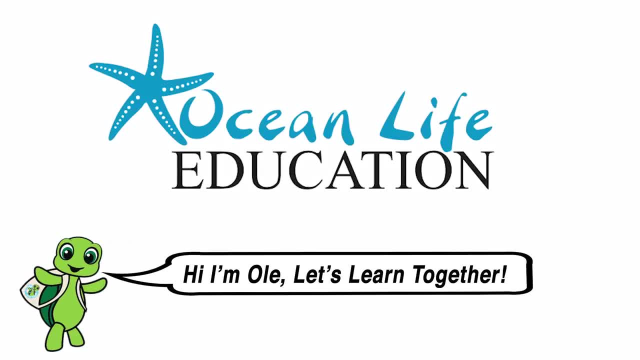 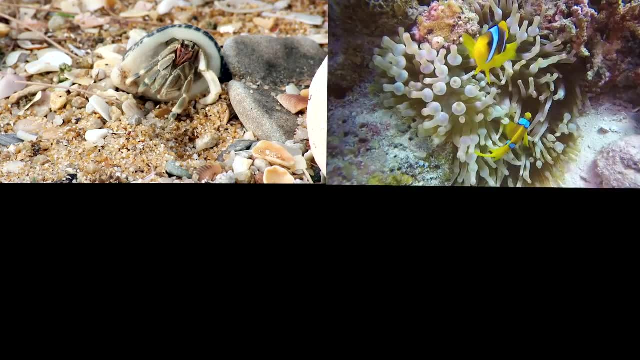 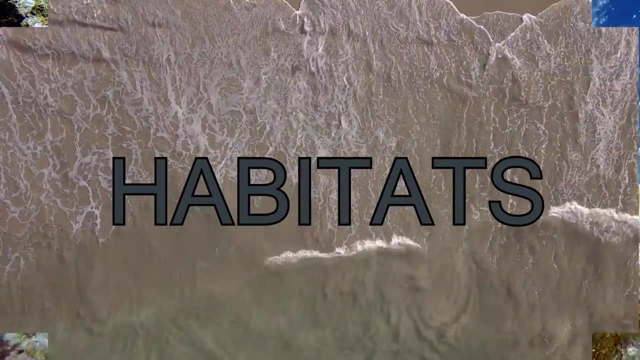 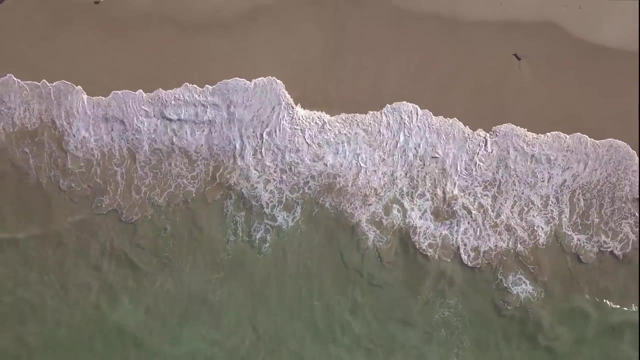 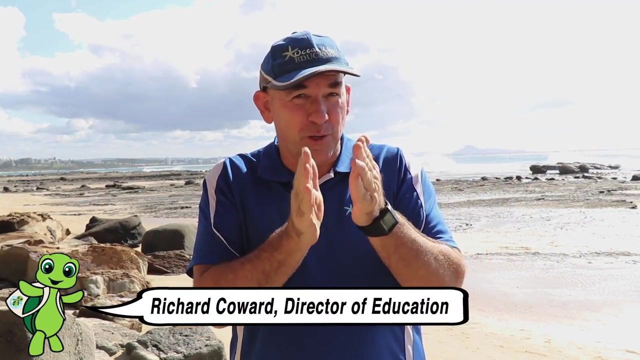 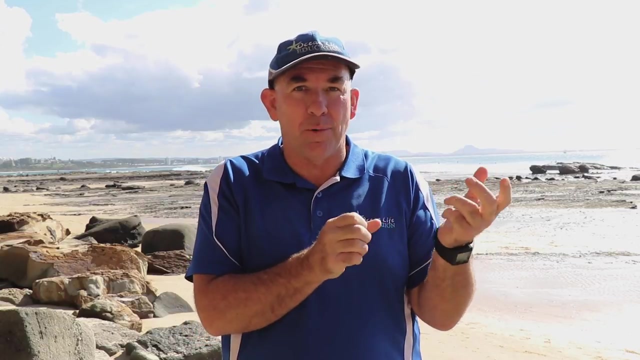 Every animal needs somewhere to live, And when an animal lives in a certain area for a certain while, that area is called a habitat. In the ocean, there are lots of different habitats. Different size animals need different types of homes, But in order for an area to be an animal's habitat, they need to find a few things. 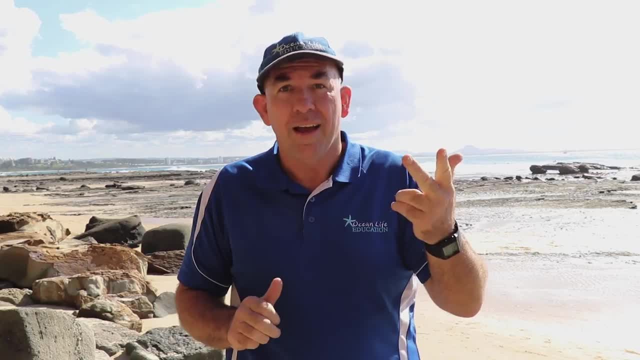 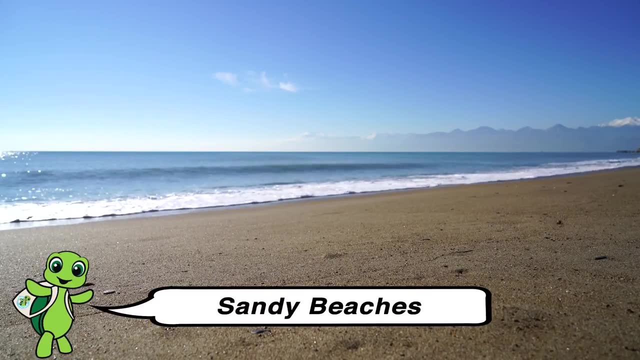 They need to find food, shelter, water and oxygen. Let's have a look at a few of those habitats. A lot of people don't realise that the sandy beaches, they're a habitat, All that sand that you see, that provides shelter for lots of different animals. that. 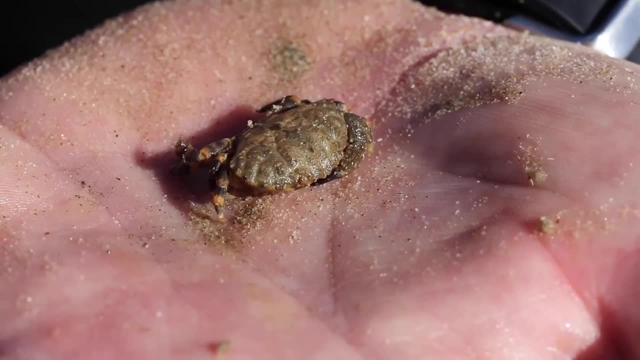 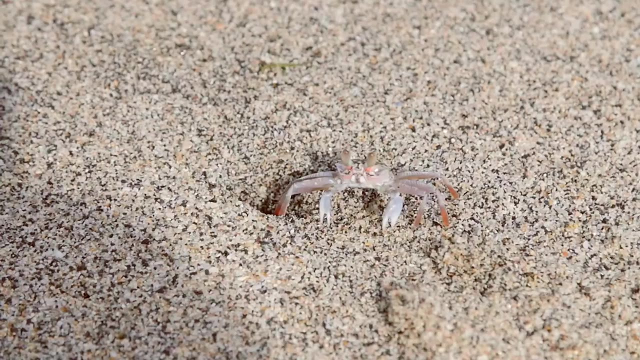 live underneath Shellfish, worms and little guys like this, crabs. They bury underneath there, then they come up on top looking for food. then they scurry back down underneath again. Really really important habitat area. It connects the ocean to the land- Mangrove swamps. 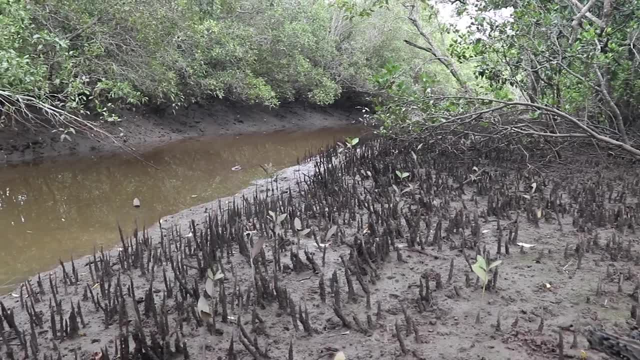 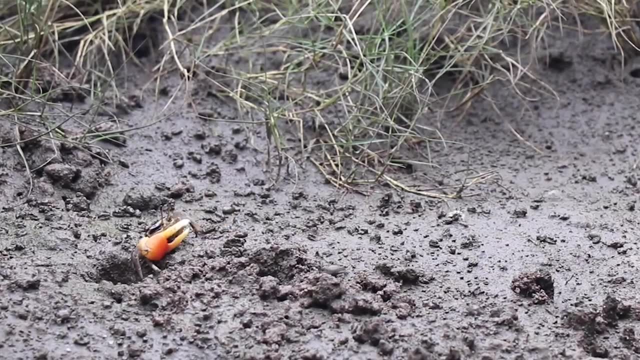 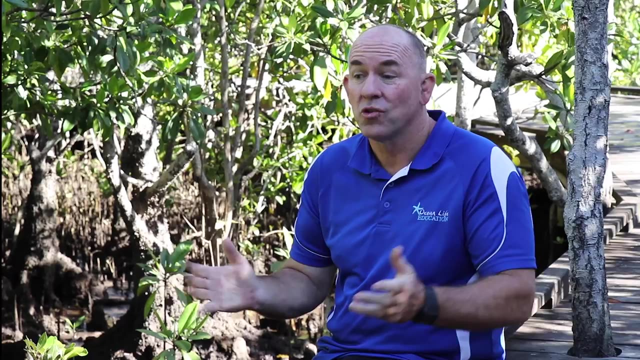 an amazing habitat area. The tree roots that come up out of the sand in the soil. they help the plants breathe when the water comes in, But it also supplies a place for animals to hide. They can hide in behind there and then they can ambush their prey, But they also trap food for the animals as well. 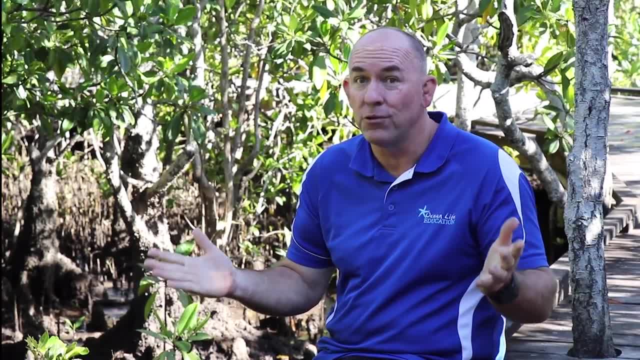 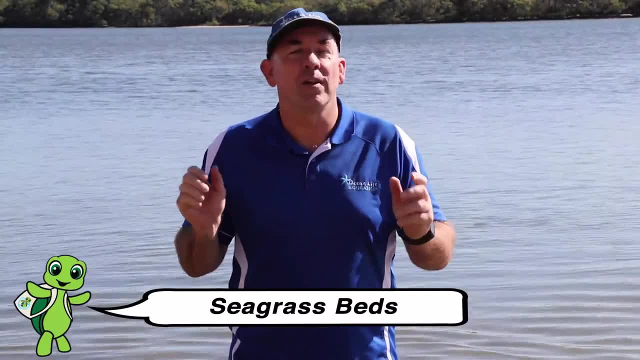 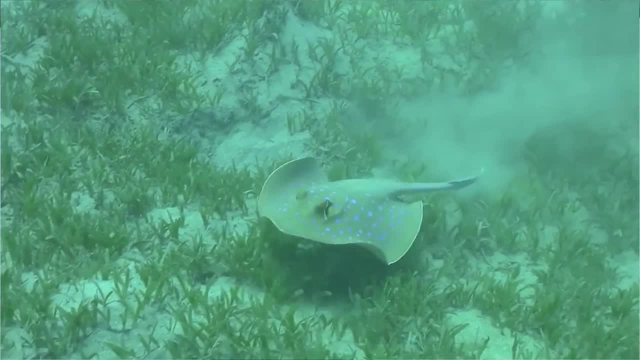 So Mangrove swamps got all the elements we need: Food, shelter, water and oxygen. A really important habitat. Seagrass beds, a really cool habitat area Usually found in shallow waters just off the coast or in rivers and canals, And in them you find some pretty amazing animals, None more amazing than 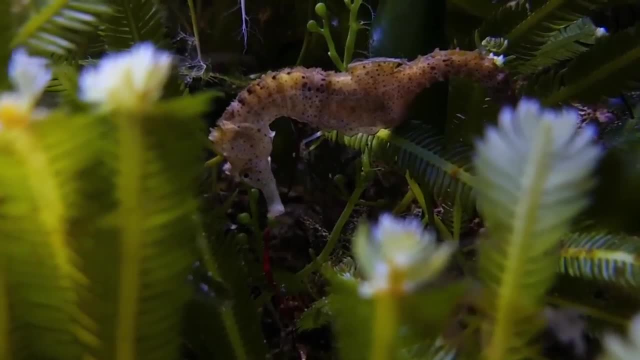 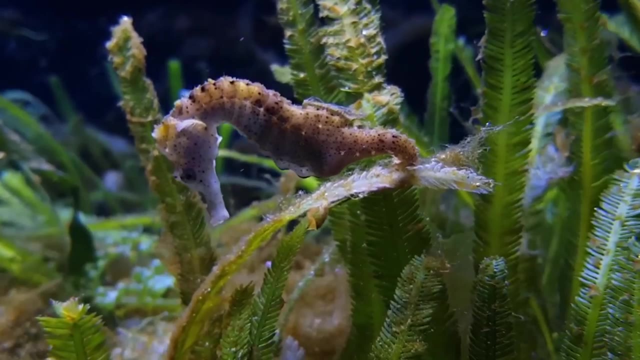 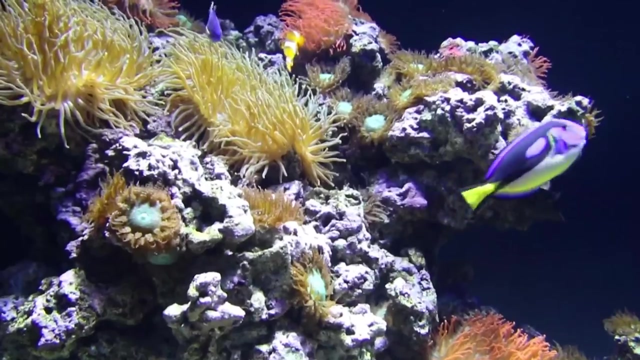 a seahorse. They actually use their tail to hold onto the seagrass, waiting for their prey to come past- Tiny little shrimps when they reach out and grab them. Seagrass beds- really cool places. Did you know that corals are actually tiny, tiny living animals And they make the coral reef?